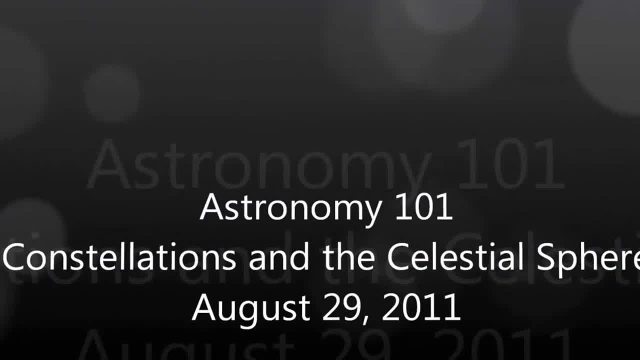 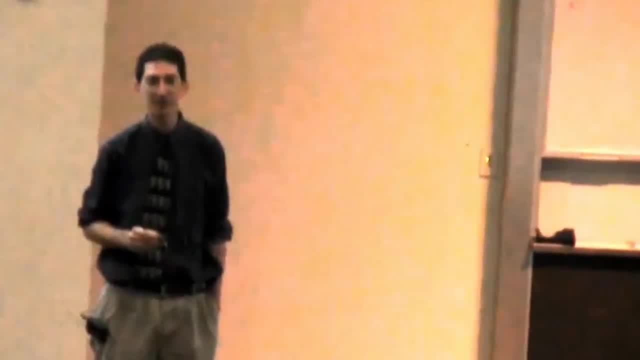 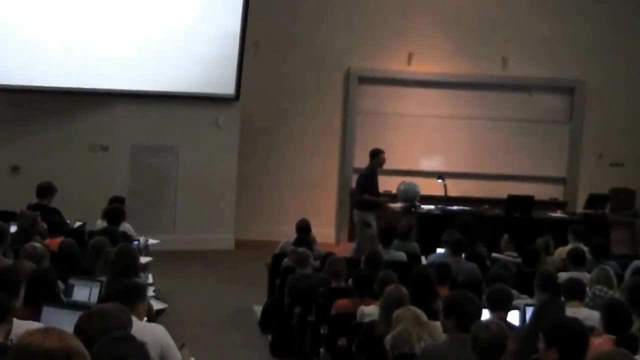 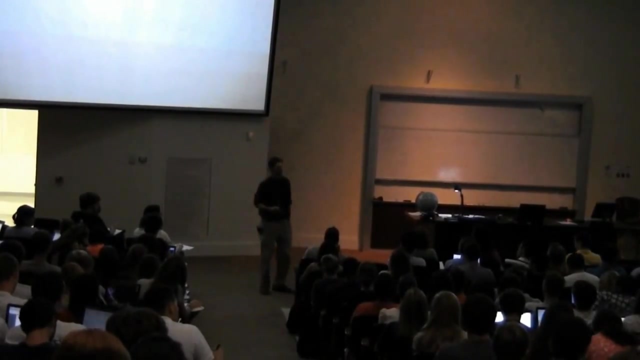 Constellations. How many of you took this course to learn the constellations? One Sucks to be you. Even I don't know all the constellations. In fact, I probably only know like six or seven constellations, And I'm a real honest-to-goodness astronomer. So there's a reason why I can. 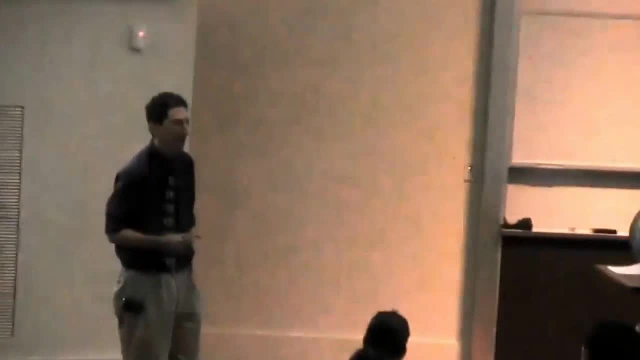 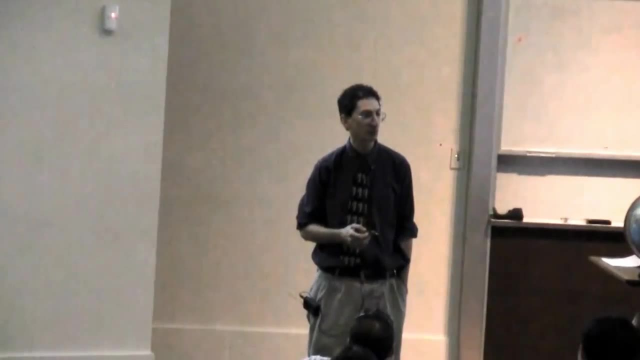 actually be a professional astronomer and not know the constellations. But back in- and we'll get to that reason in a second- but back in the day, astronomers knew the constellations. There's a very practical reason for knowing the constellations Anyone want. 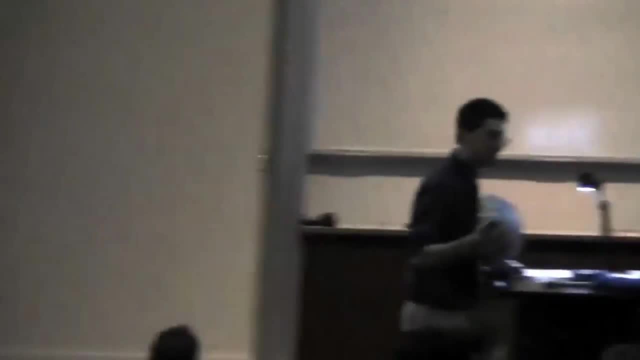 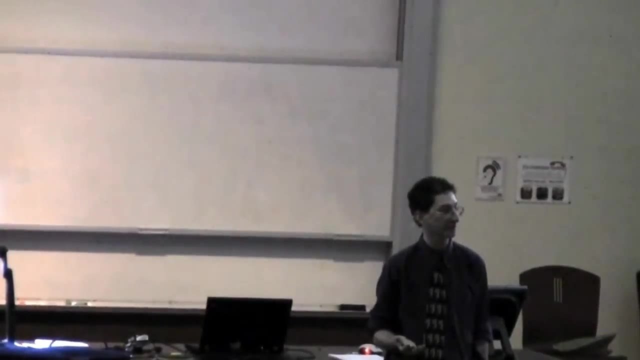 to venture a guess, Navigation. So if you're sailing a ship, knowing the constellations and the stars and having an understanding of the sky was crucial. We all know there's one star that kind of points to the north always. We call that star Washington. 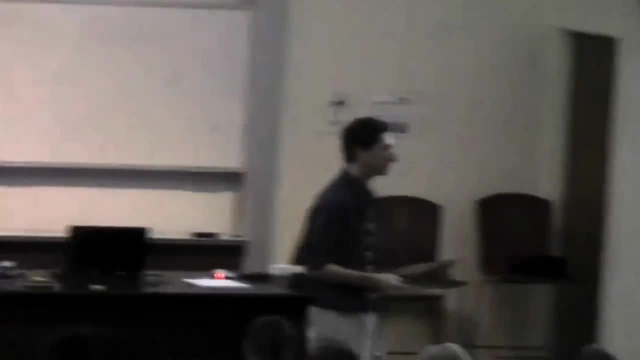 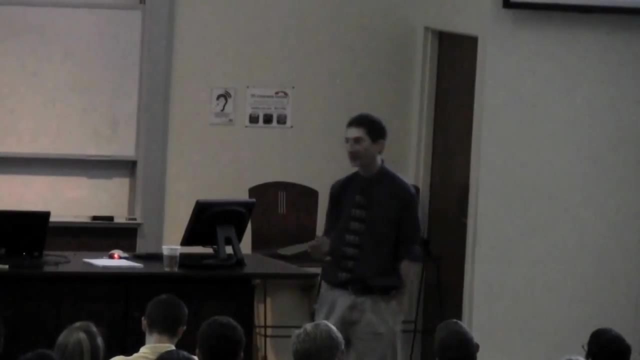 What Polaris? Polaris, You can navigate off of it, Even if you don't see Polaris. if you're in the southern hemisphere, if you understand how the stars are moving, the various constellations, you can use it for navigation of ships. But astronomers aren't, weren't? 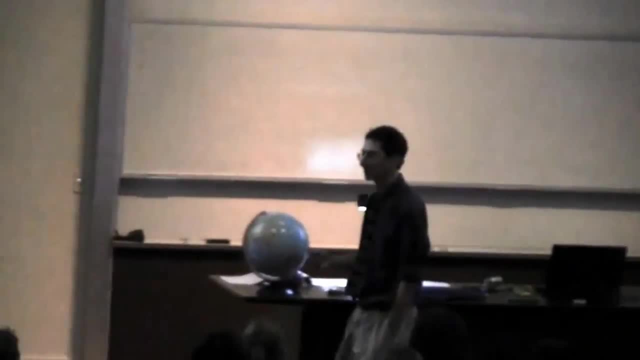 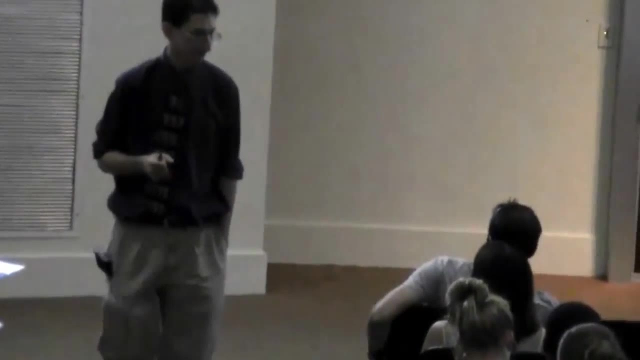 called on to go on every sea voyage to help keep the ship where it needs, you know, on the path it needed to go. Astronomers need to understand constellations for a reason too: How were they? Where were they in the sky? It was the way it was harvested. 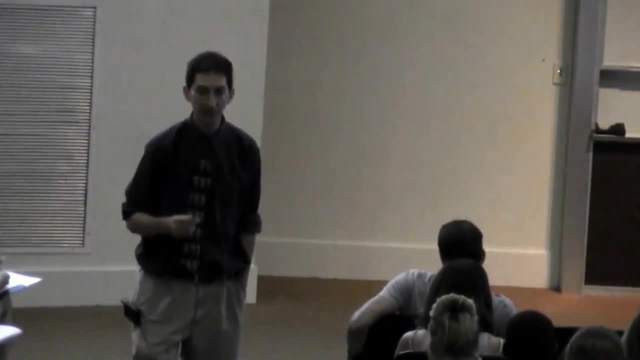 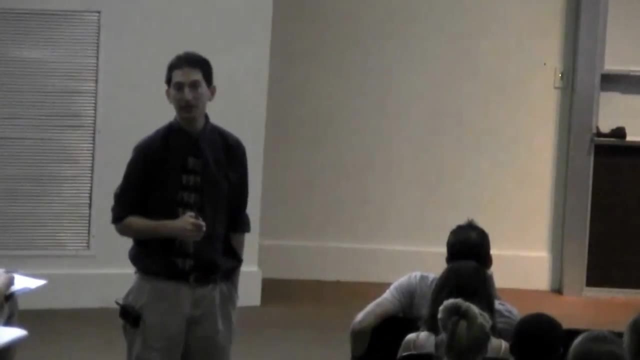 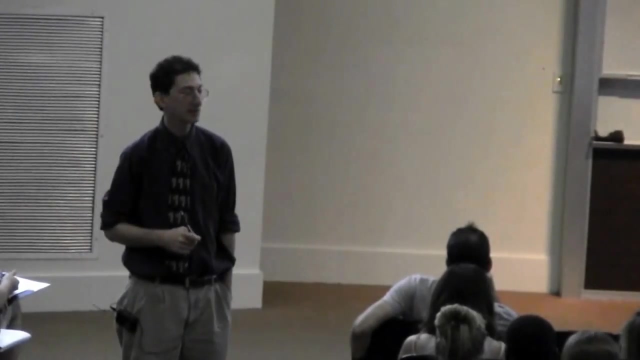 That's right, We so, she said we use them as a calendar and we'll get to that. Particularly as we begin lesson two, you'll see, going back to even prehistory, the stars and objects in the sky were used as a basic calendar as well. But just to be a practicing astronomer, 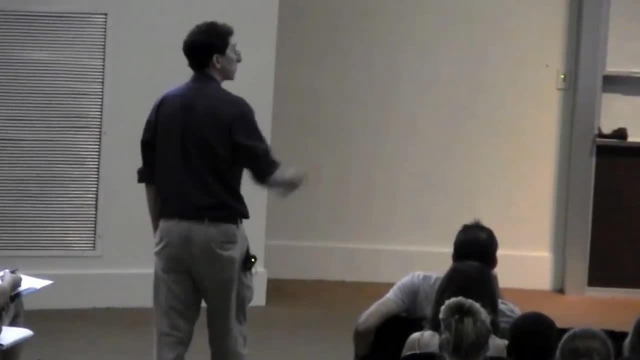 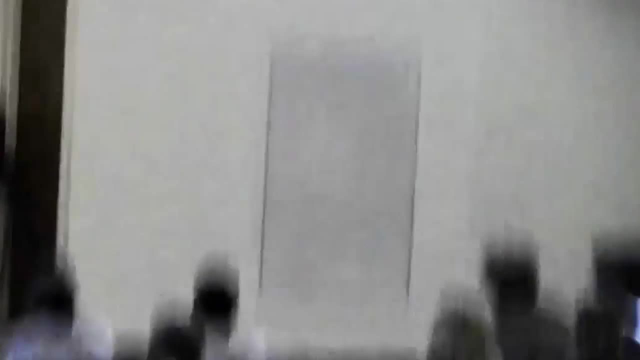 it's useful to know the constellations because suppose, suppose one of these stars here was acting up. Let me pick one. Maybe this little star right there, Maybe it's getting brighter and fainter and brighter and fainter. As an astronomer, you 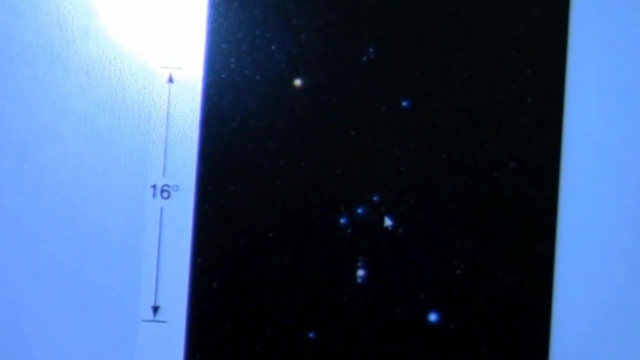 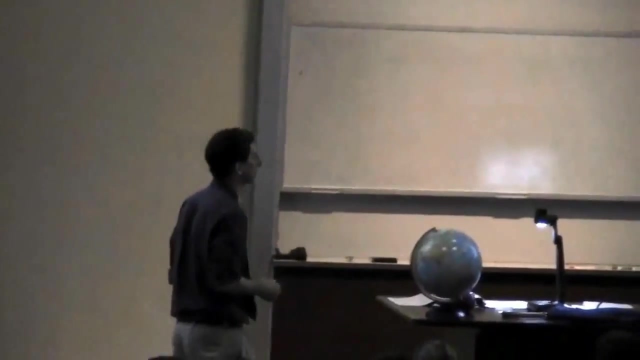 know most people don't care, but as an astronomer I'm excited. Maybe it's going to blow up, Maybe who knows what it's going to do, And I want to report that to my colleagues elsewhere around so they can actually look at the star and confirm that I'm not crazy, and maybe their 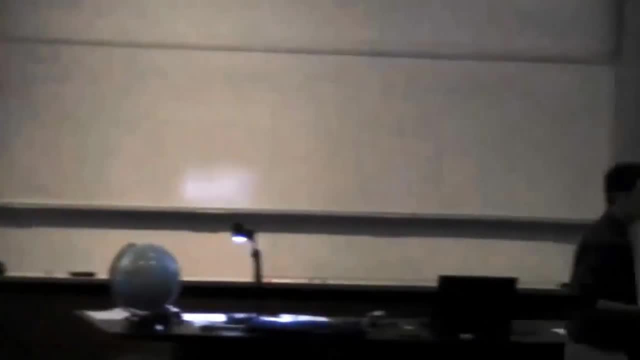 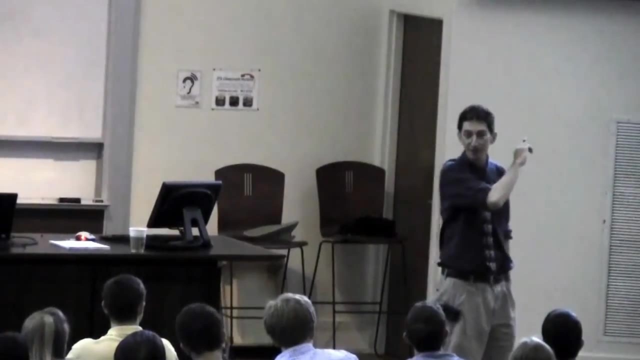 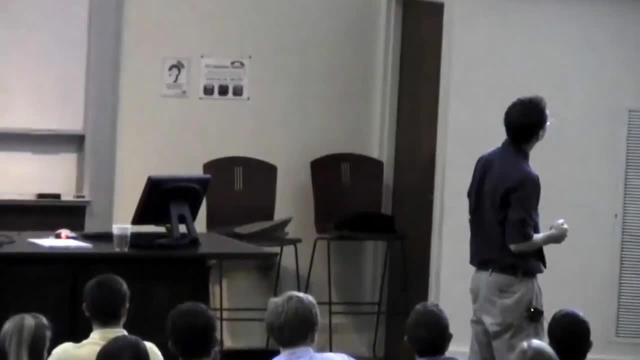 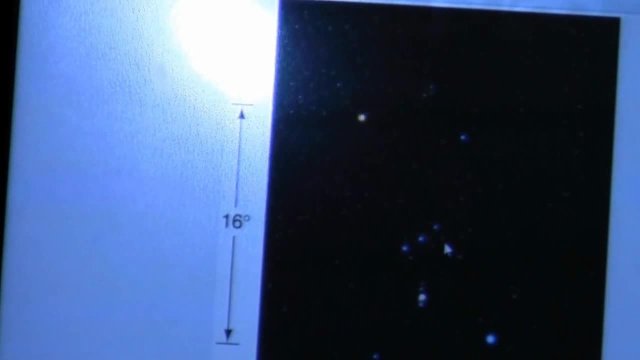 Arunachalaka, Arunachalaka, Arunachalaka. And then go to the belt, go to the kind of the top of the belt and then go diagonal from that topmost star towards the blue star in the foot. Rigel, The big blue star is Rigel. 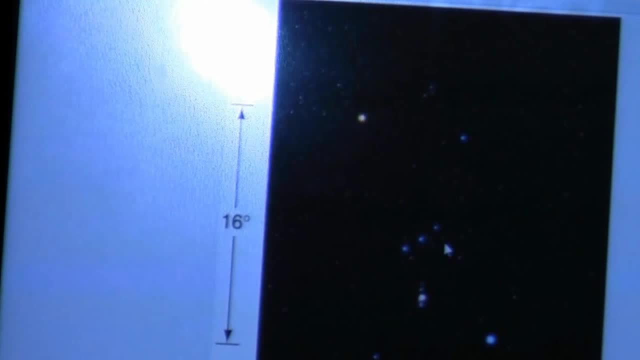 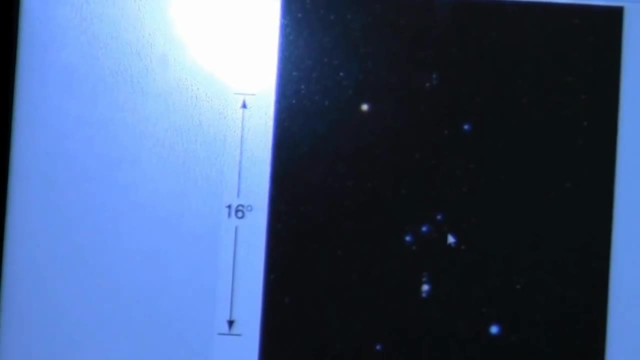 the big red star is Betelgeuse, So go in the direction of Rigel just a little bit and there's the star I'm talking about. So it's a way to navigate the sky, let others know that there's something important going on there. 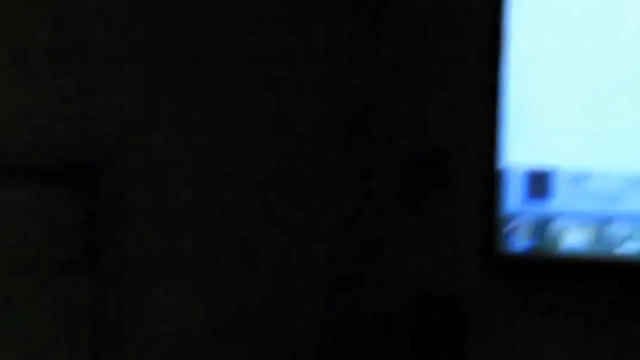 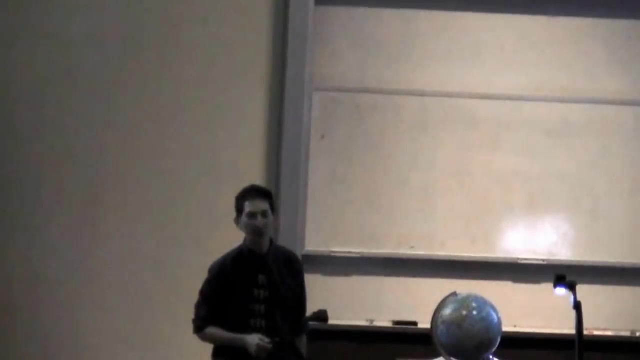 So, but nowadays you know that was a really good idea. So, but nowadays you know that was a really good idea. That was useful back then, but nowadays we don't navigate the sky that way, particularly because often we're looking at stars that are too faint to even see with the human eye. 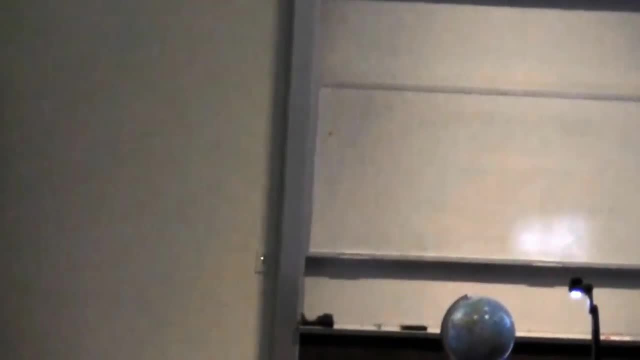 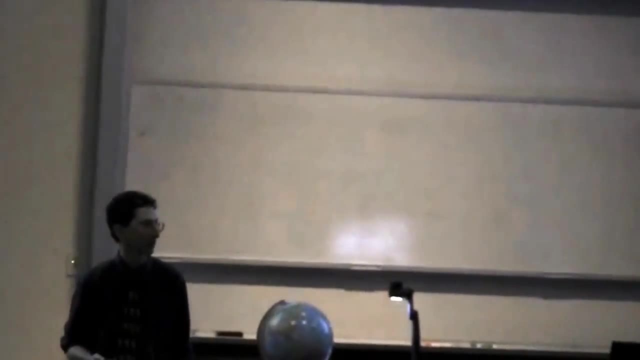 and sometimes we're navigating the sky in wavelengths the human eye doesn't even work at, like radio or x-ray or gamma ray, So in the modern era we have to rely on what- What do we call it- To navigate the sky: GPS. 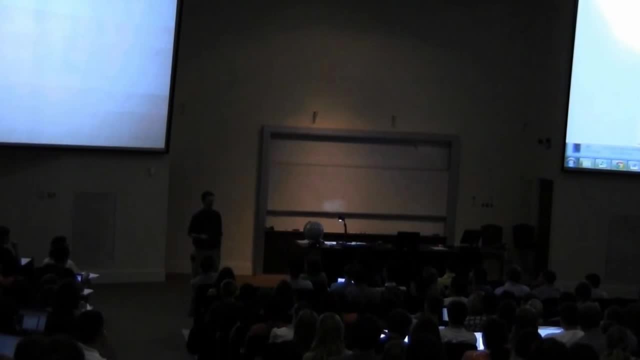 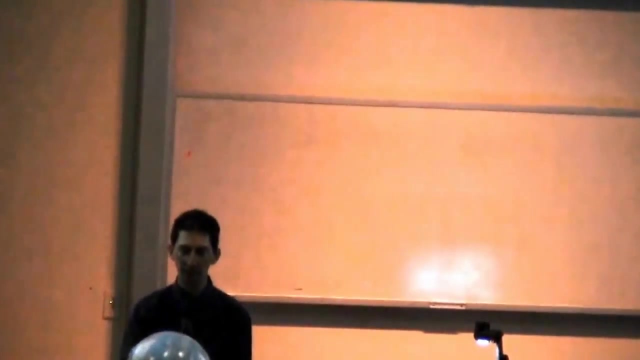 That's actually very much related. GPS is giving us what Coordinates, yeah, And so astronomers have a coordinate system for the sky, just like on Earth we have a coordinate system that the GPS uses, and the two are intimately related. So here's a globe, and so this is a representation of the Earth. 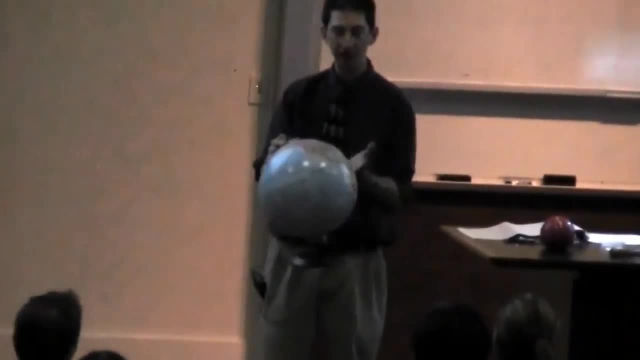 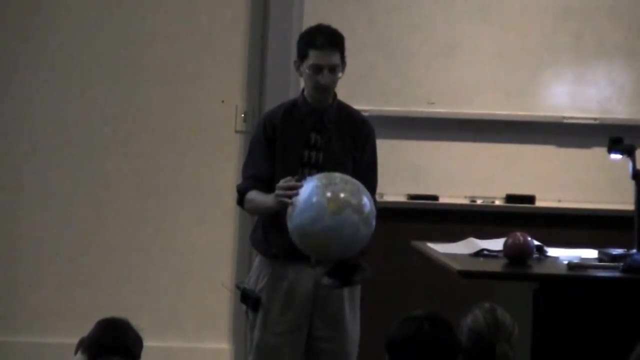 and there's a coordinate system on it. You may not be able to see it from your distance, but there are lines going around it this way and lines going on it this way, a two-dimensional grid on the surface of the sphere, and we call that a coordinate system. 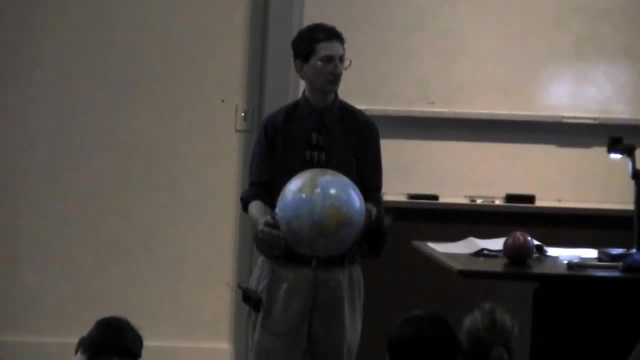 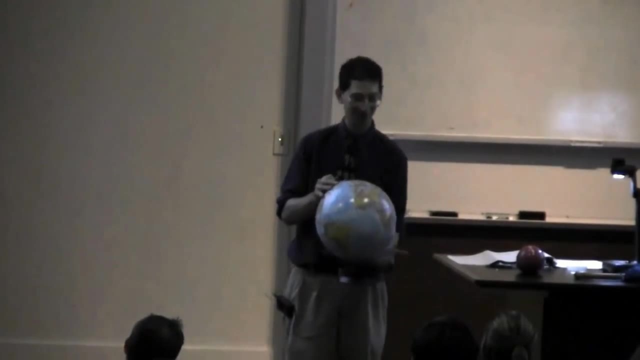 What are the two coordinates called The globe, Latitude and longitude, Which one runs from pole to pole. Latitude: Latitude changes up here to plus 90,, down here to minus 90, and you have 360 degrees going around the Earth in this direction. 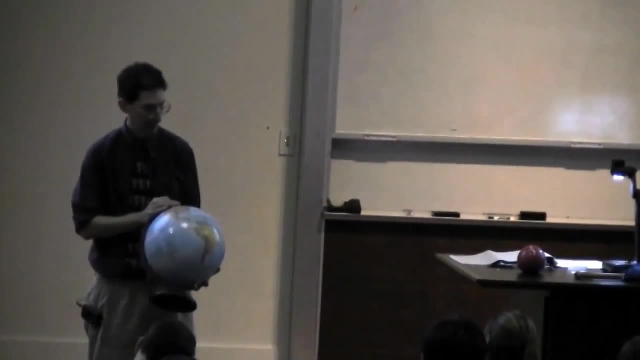 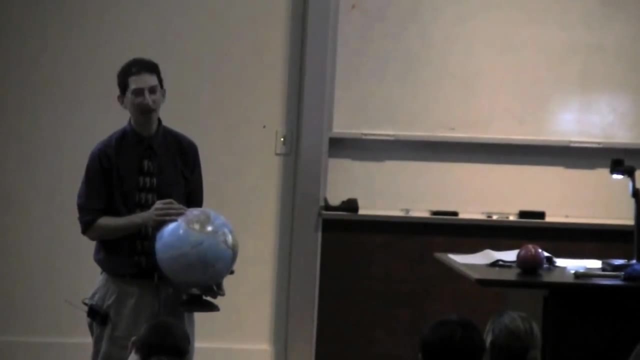 Well, we can do the same thing for the stars in the sky, and it's based upon our lack of understanding of distance. Like when you look up at the sky at night, can you see how far the stars are from us? No, 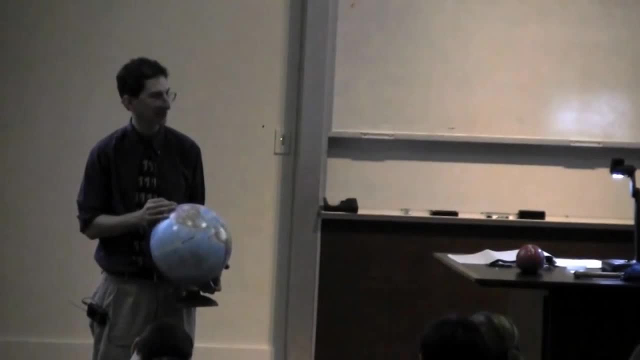 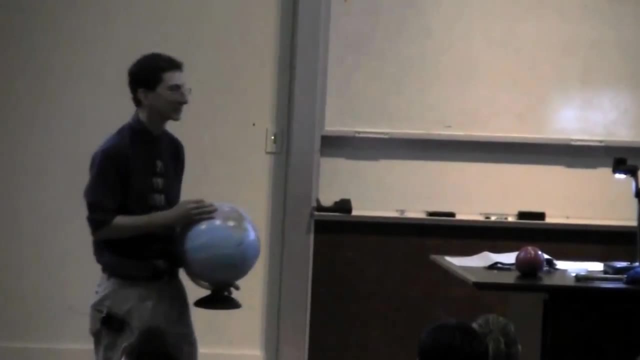 We have no idea how far they're away. Distance is the hardest thing to measure in astronomy. We have to use all sorts of tricks to figure out distances. Just looking at the sky, we have no comprehension of distance or that some stars are farther away than others. 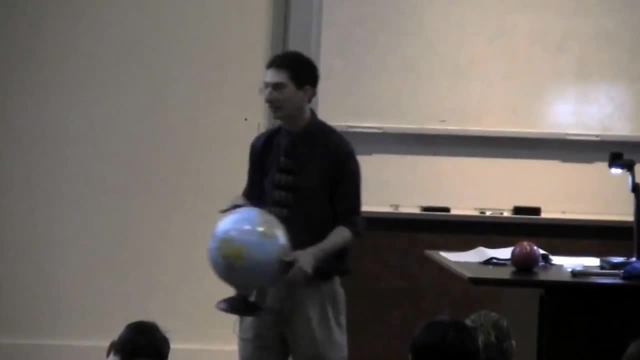 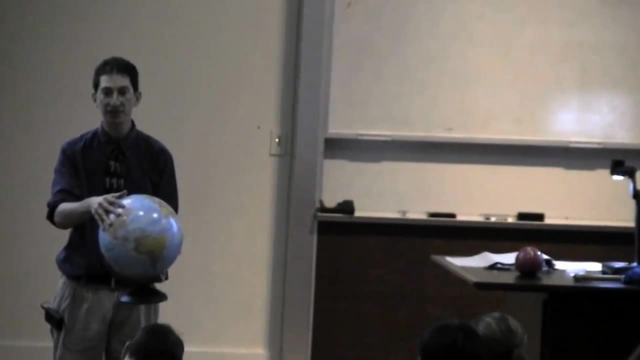 They all appear to be kind of at the same distance. In fact, this is what the ancient models, cosmological models, assume. The ancient models assume Earth is sitting here at the center, and then around it there is a sphere. They didn't think of the stars as distributed through three-dimensional space. 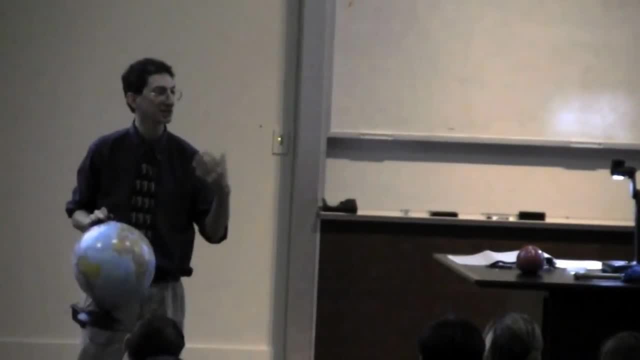 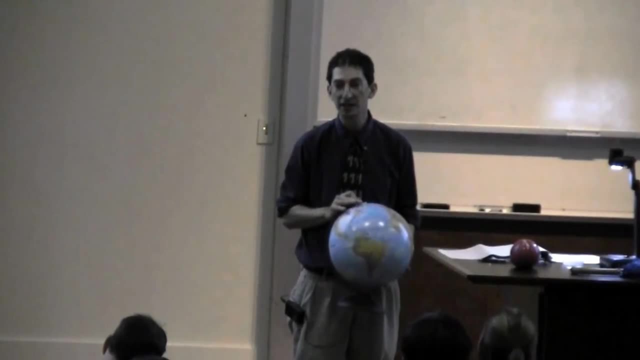 They thought there was a sphere that encompassed and closed the Earth. They called it the celestial sphere. It's still useful today as a mental construct, and we're trying to talk about how the sky appears to move If you're standing underneath it. 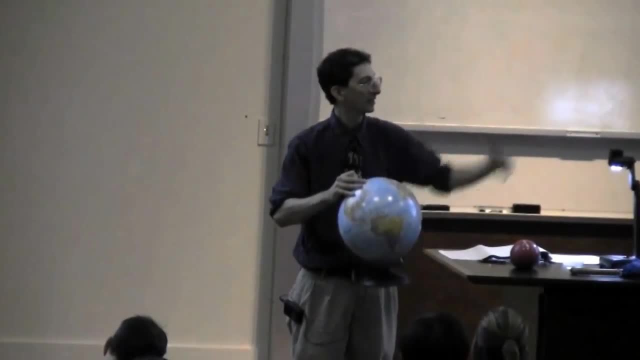 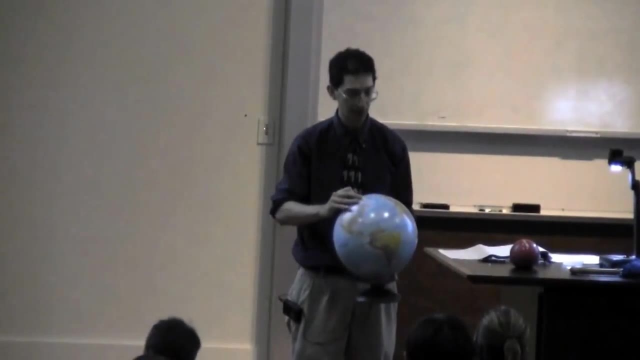 we often talk about the celestial sphere, even today, But imagine the sphere encircling the Earth. You can do that. Since we can't see distance, we can pretend they're all at the same distance, painted onto this sphere. And 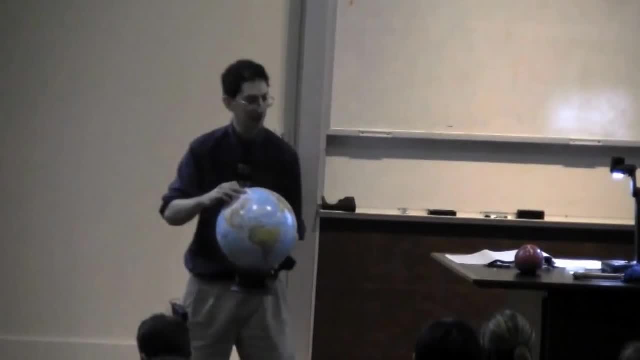 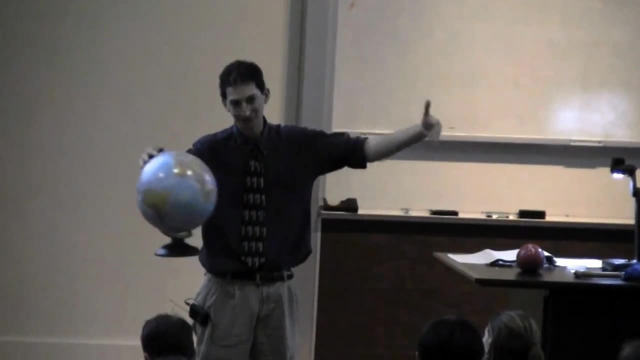 You know the The. You know, back then they thought the Earth was standing still and the sphere would actually go around the Earth. The whole universe would go around us. Nowadays we know that well, under the idea of the sphere, the universe is out there. 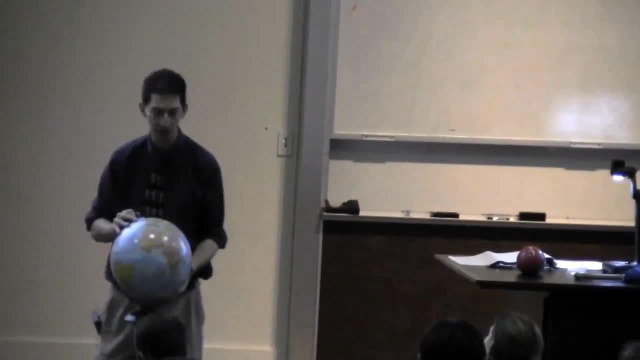 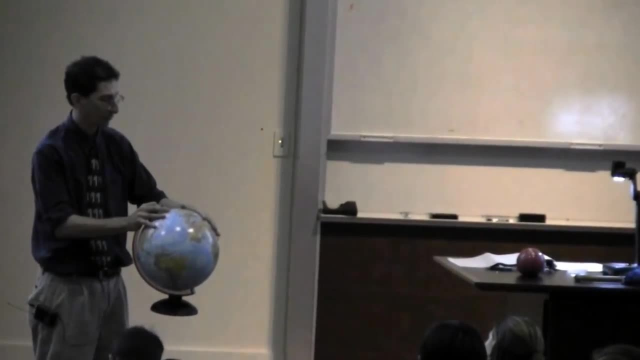 and we're rotating underneath it. It makes the appearance of motion of these stars. But that aside, imagine taking the coordinate system of the Earth, the longitude-latitude coordinate system, and projecting it out kind of from the center of the Earth. 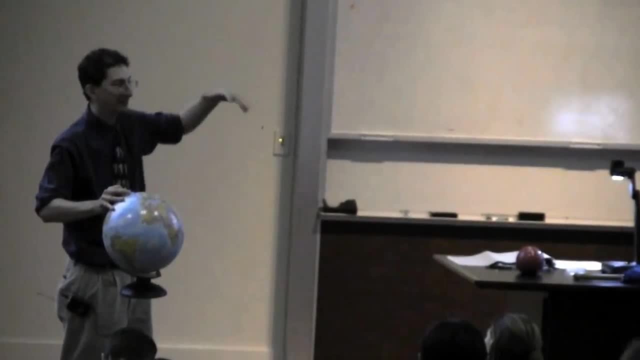 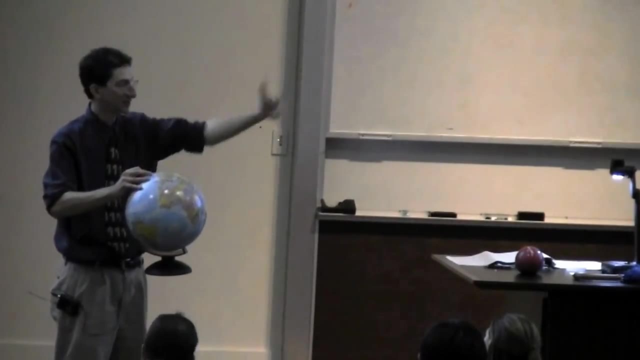 radially outward onto the celestial sphere and then fixing it to the sphere. As I just said, you can envision the Earth standing still and the sphere moving, or you can envision the sphere standing still and the Earth moving, But in either case, 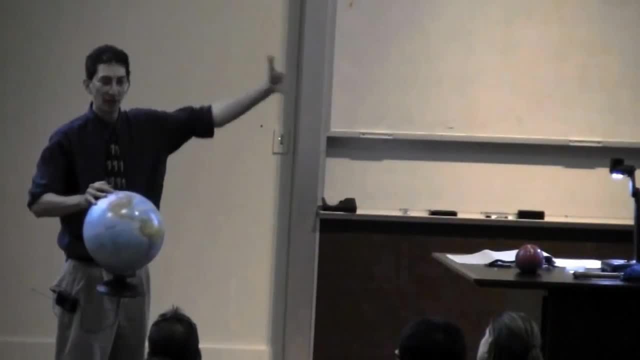 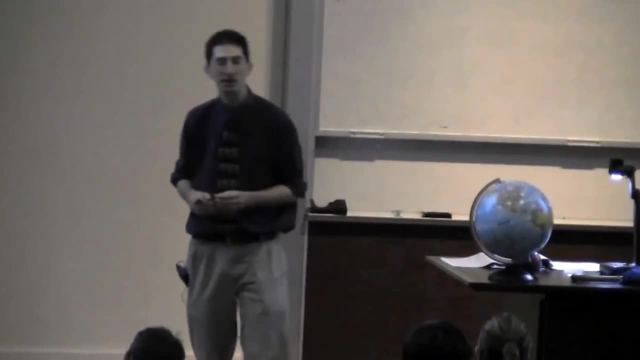 the longitude-latitude coordinate system is fixed to the Earth. This other coordinate system is fixed to the sky And we don't call those coordinates longitude and latitude. but what do we call them if we're talking about the sky, Declination and right ascension? 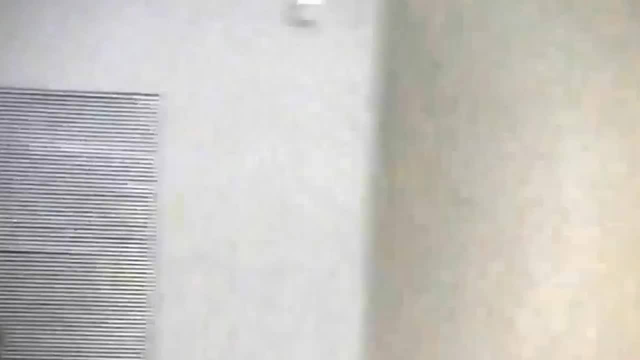 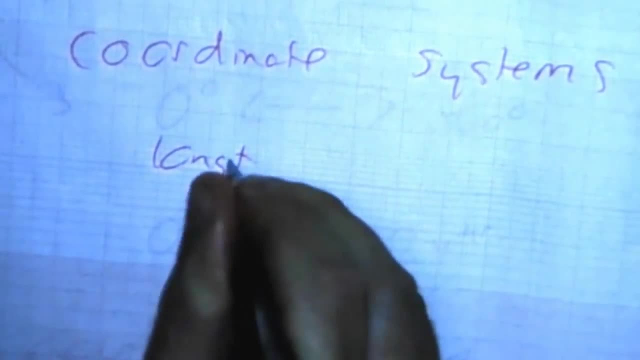 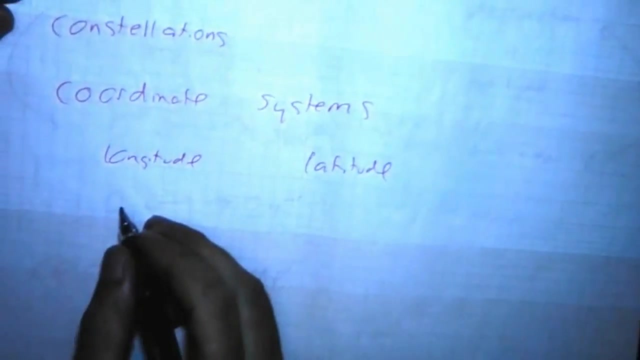 So let's make a note here: This is coordinate systems. So on the Earth we have longitude, longitude, latitude, And on the sky we have um, which one corresponds to longitude, Right ascension or declination. 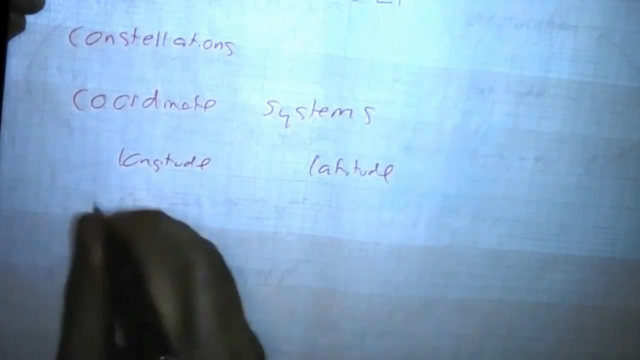 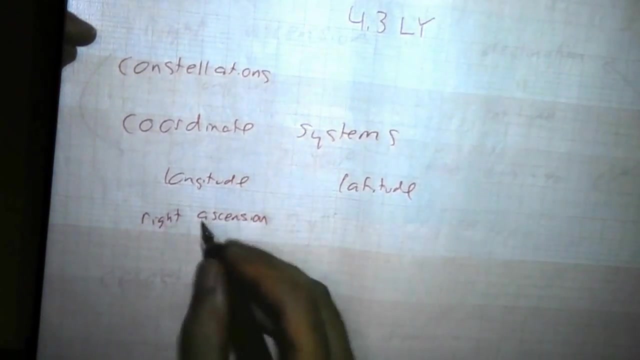 Right ascension, Right ascension- It's a weird term, but that's what it's called. You can just think of it as longitude for the sky. Latitude, we call that declination When fixed to the sky. When fixed to the sky. 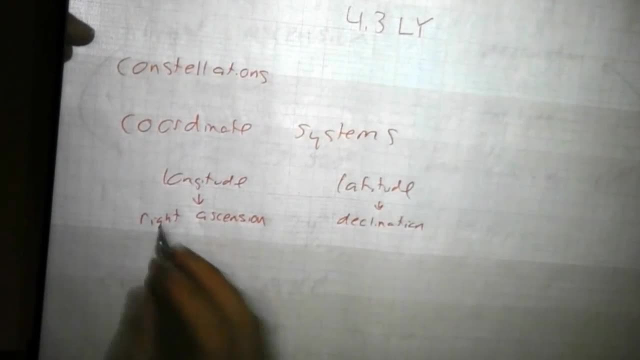 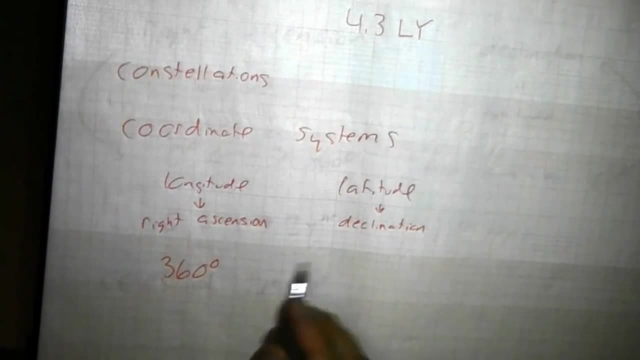 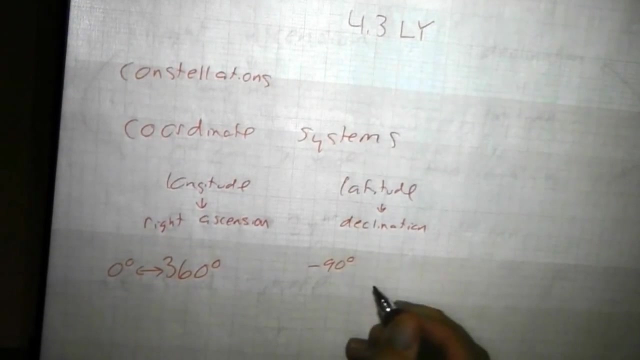 we have 360 degrees going around the sphere, So 0-360 degrees And latitude. we go from minus 90 degrees in the South Pole, whether it's the South Pole of the Earth with latitude or the South Pole of the celestial sphere. 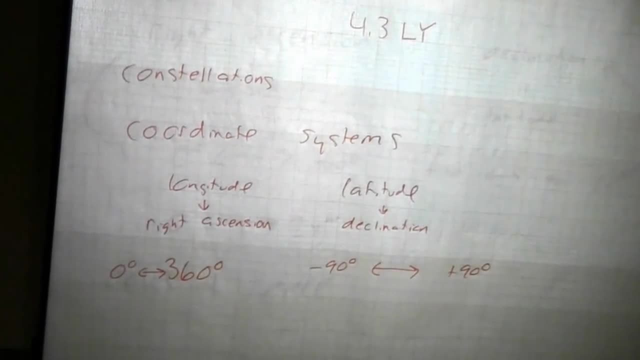 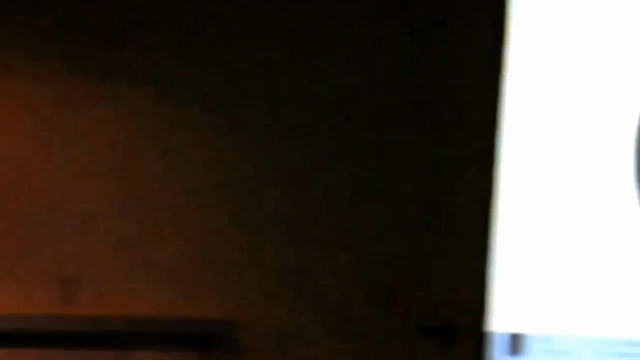 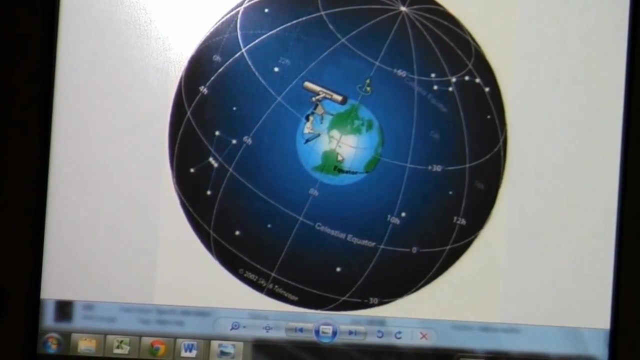 to plus 90 degrees at the North Pole. So here's a figure to illustrate that. So, just as I was kind of waving about with my hands here, we've got the Earth in the middle, this mental idea, construct of the sphere encompassing us, and we have coordinates on it. 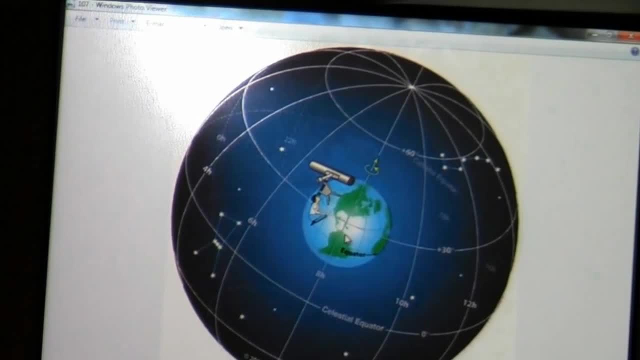 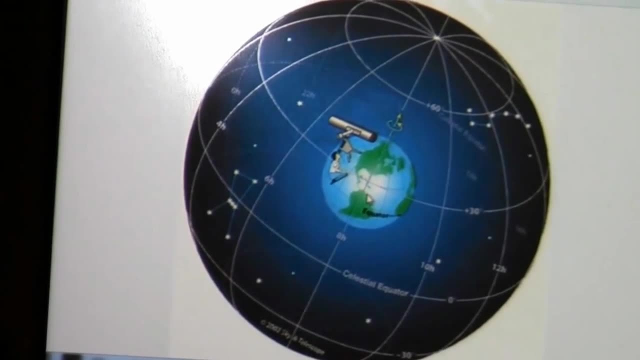 We've attached it. You can see the longitude-latitude coordinate system. You can see it projected and drawn on the sky. Now they rotate with respect to each other, but the one on the sphere rotates with the sphere and with the stars that are painted on the sphere, so the stars are kind of fixed with respect to it. 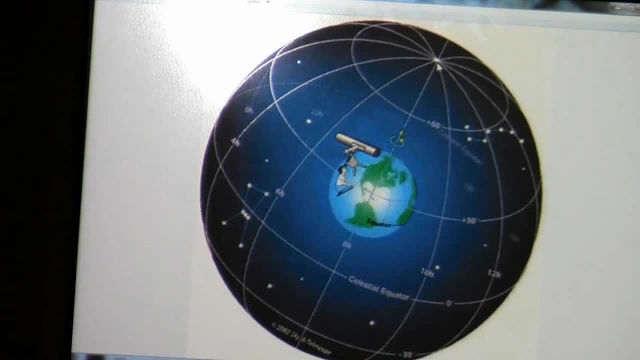 And you can see the numbers here, We've got the pole up here- would be plus 90, declination plus 60, plus 30.. Zero is the celestial equator, which is just a projection of Earth's equator onto the celestial sphere. 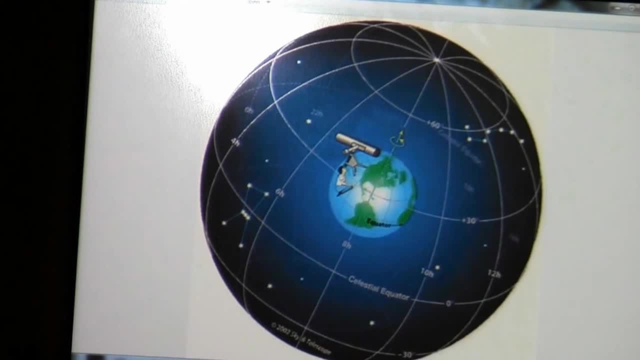 Going down we've got minus 30, and then below we can't see it, minus 30. I'm sorry, minus 60, and then minus 90 is the south celestial pole. It's like we call that the south pole. This is the south celestial pole. 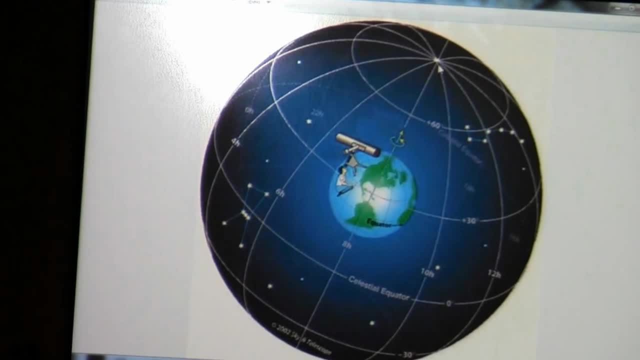 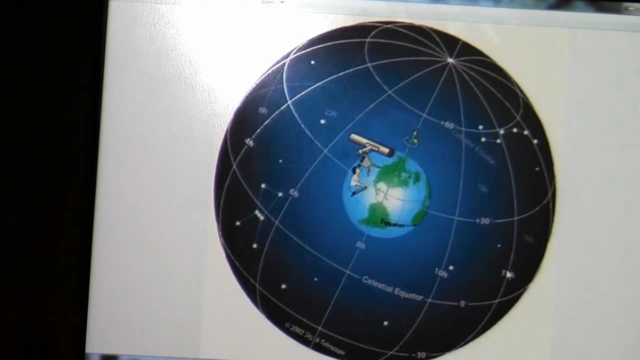 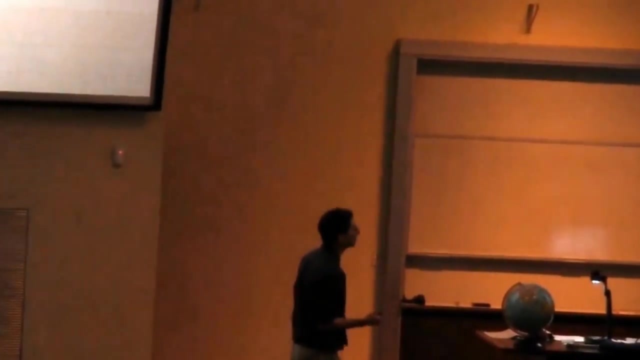 North pole, north celestial pole And going around the celestial sphere. the longitude goes from 0 to 360 degrees. Right ascension can also be described that way: 0 to 360 degrees. So there's kind of a convention in astronomy that the right ascension instead of using degrees we use hours. 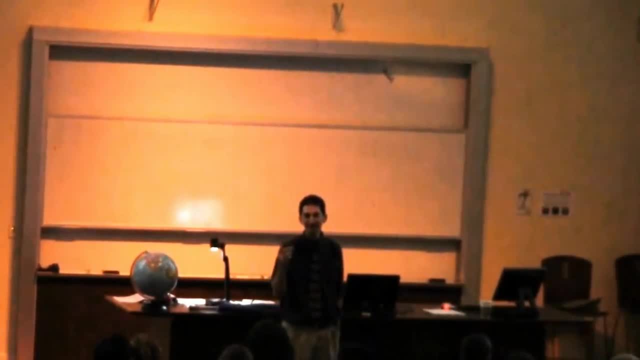 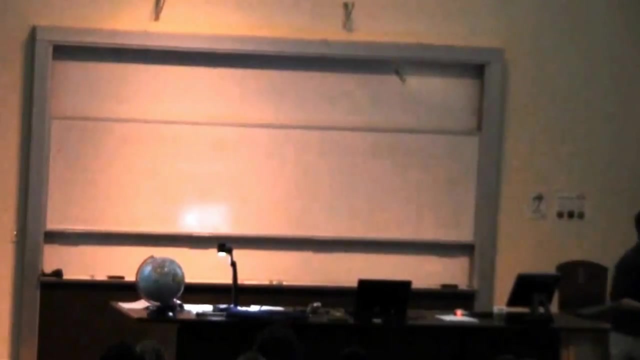 Because in one day, the celestial sphere appears to rotate. how many hours? 24, right, Because the Earth is spinning. It's spinning on its axis once every day, once every 24 hours. So from our point of view, it's as if the celestial sphere is spinning around once every 24 hours. 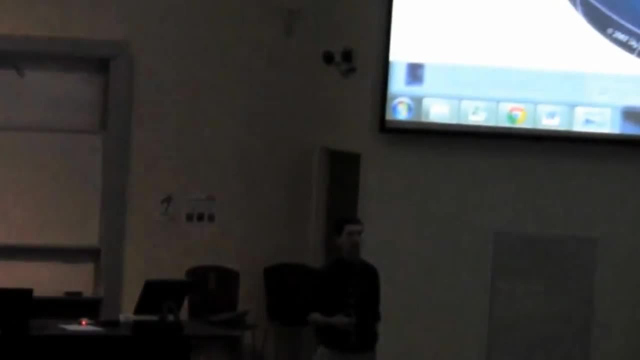 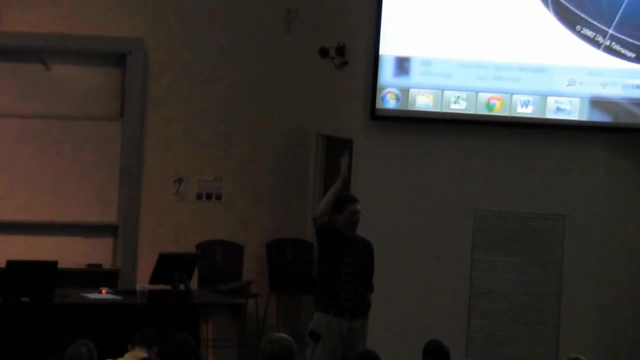 So instead of using degrees, the historic convention is to use hours. So if there's a star above you at one hour right ascension, in an hour the stars at two hours right ascension will be above you. In another hour, the stars at three hours right ascension will be above you. 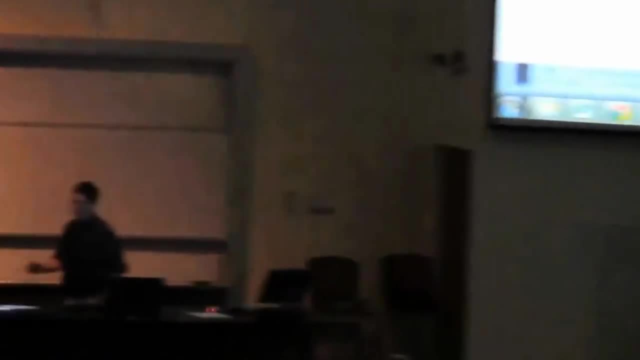 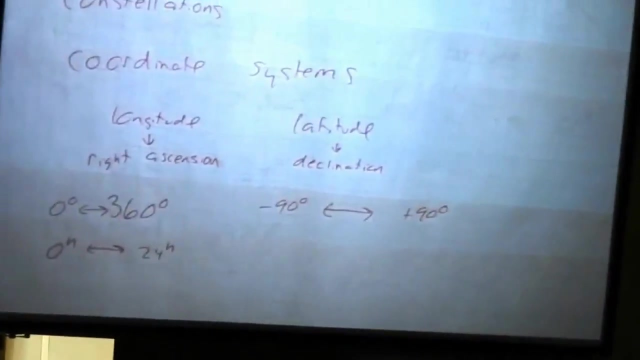 So we just use hours. It's kind of convenient. So right, ascension can be 0 to 360 degrees or 0 hours to 24 hours, and then 24 hours is the same as 0 hours. Now, we're not going to make use of that in this course. 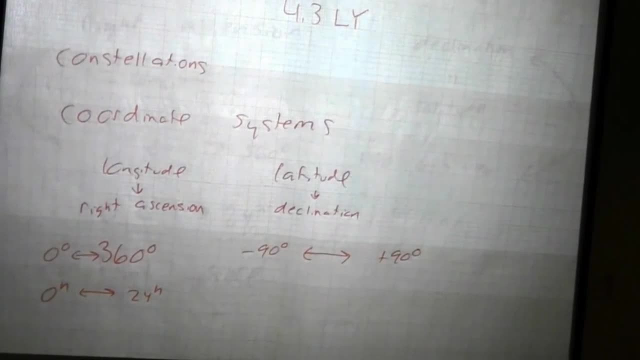 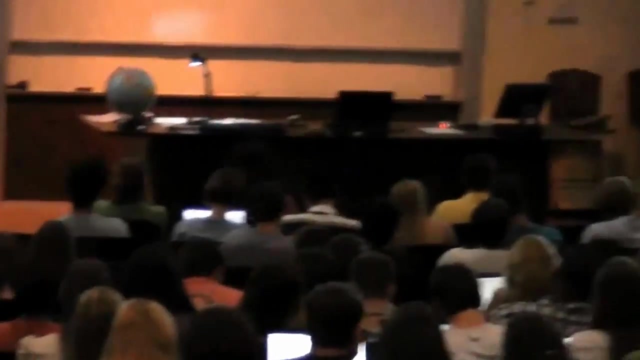 though, if you're taking the lab and you're scheduling observations on Skynet using the Prompt telescopes or some of the other Skynet telescopes, there are boxes where you input the right ascension and declination. Though it also makes it easy, We do live in the modern era. 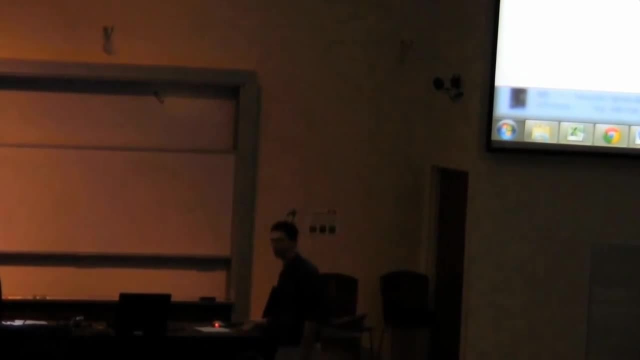 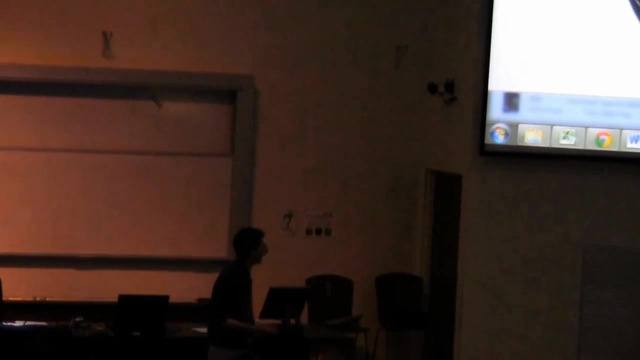 If you want to look at Jupiter, you don't have to go to some book and look up the coordinates of Jupiter at this point. You just type in Jupiter and Skynet will look up the coordinates for you. So you can actually go through the labs without having too deep of an understanding of right ascension and declination. 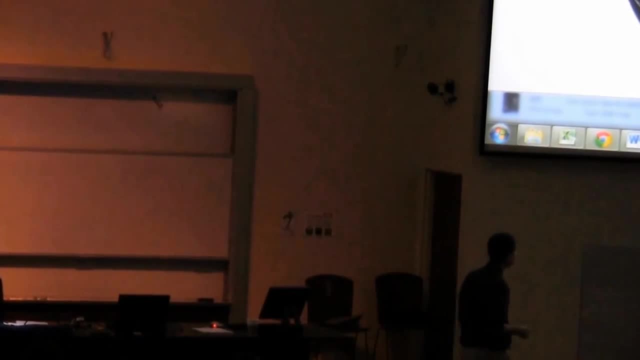 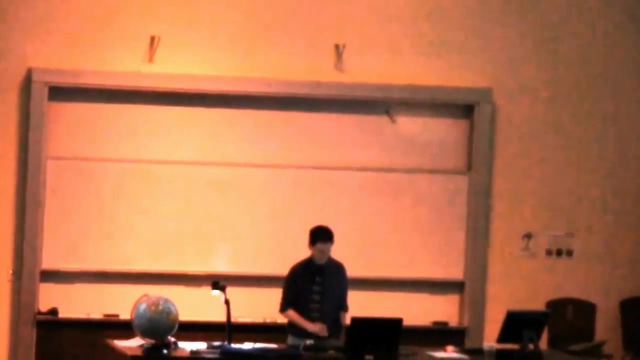 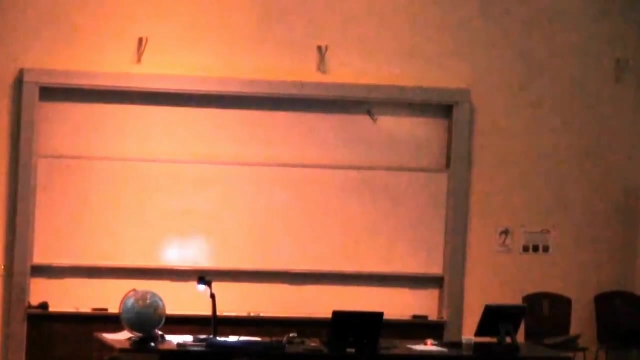 But I just wanted to give you a little bit of it right now, at least for those of you in the labs. But it's a coordinate system. Okay, So that was a tangent. Let's get back to. Oh question: A coordinate system which may be relative to Earth. Sort of like You were saying: what do you mean by a planet? Could it be Earth? So the question is: is the coordinate system with respect to Earth? If we went to a different planet, would we need a different coordinate system? And the answer is yes and no, It depends. The stars are so so far away that if we hop from Earth to the Moon or to Mars or to anything in the solar system, the distant stars aren't going to appear to shift, hardly at all, because they're just so far away. 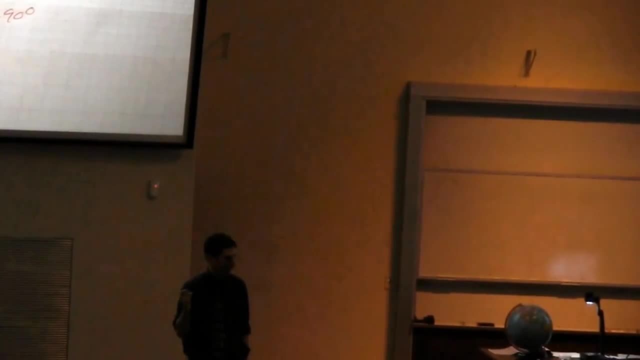 Maybe the nearby stars, like Alpha Centauri, might shift a little bit. In fact we see shift of its position when Earth moves from one side of its orbit to the other. It's a parallax effect, something we'll get to a little bit later. 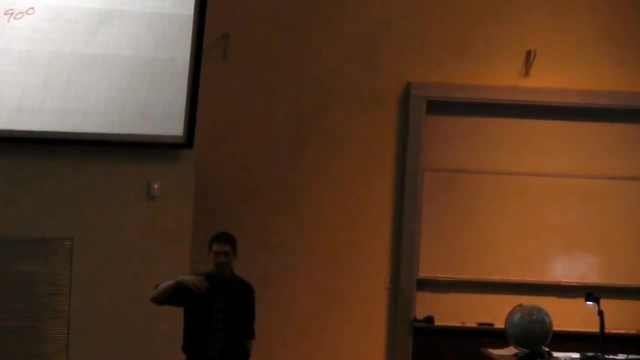 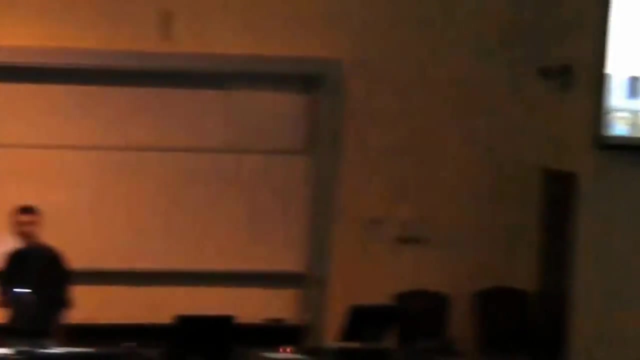 Now, if we were to go to different stars, particularly far away in the galaxy, then all the stars will appear to shift their position, So it really is an Earth-based system. Good question, Okay, Constellations, Oh, another question Good. 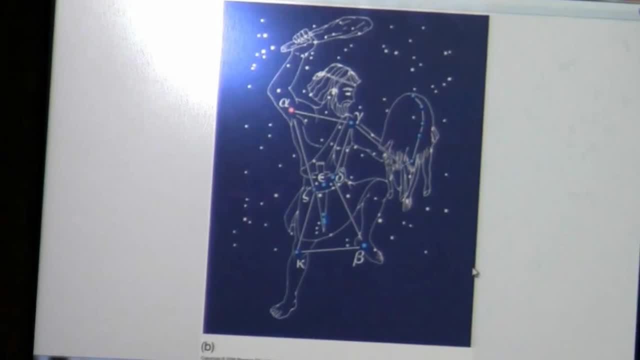 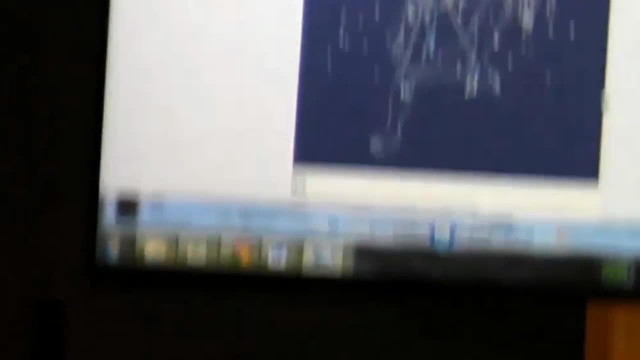 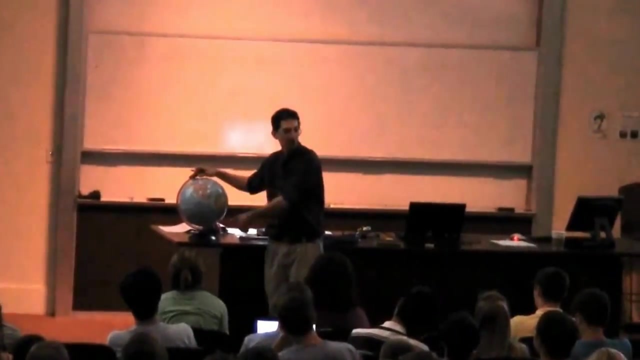 Is the celestial equator different from the ecliptic? Is the celestial equator different from the ecliptic? And the answer is yes. The ecliptic is the plane of our solar system. So you can see, here the globe, Our Earth, is tipped just a little bit. 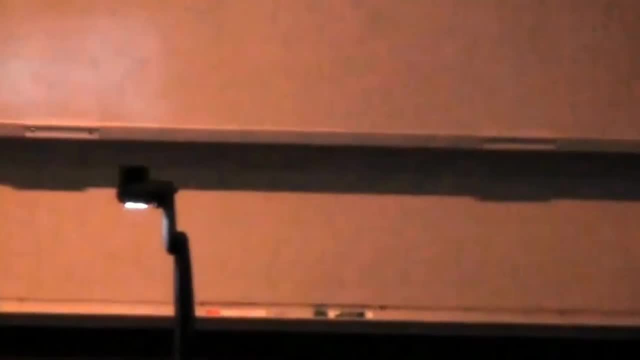 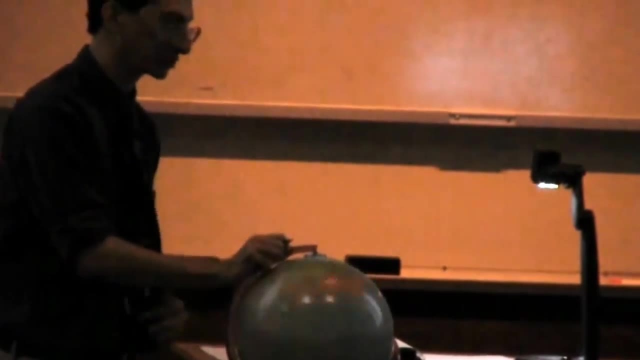 It's because, Well, when we formed, Let's say, this is the plane of the solar system, The desk, the sun is maybe my laptop- When Earth formed, it was almost certainly pointed straight up and down. All the planets were. 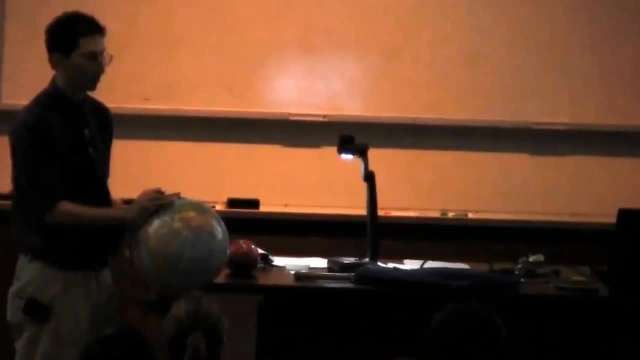 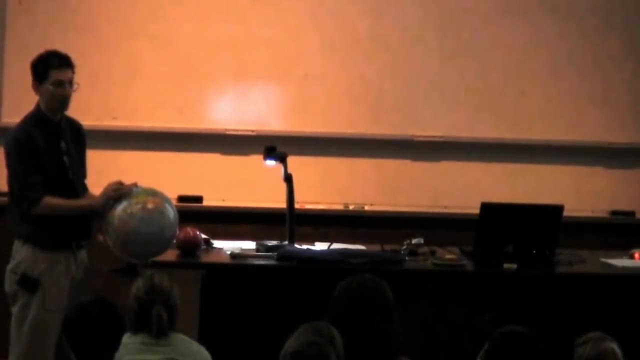 But the early solar system was a mess. It probably formed twice as many planets as we have nowadays. We had a lot of collisions. Earth was probably struck by something about the size of Mars in its early history, Tipped it over And some of the debris that came off formed the Moon. 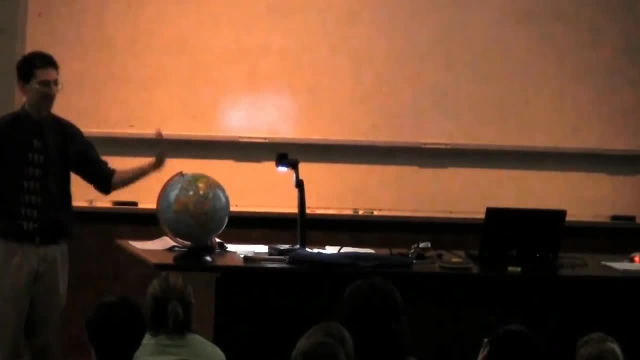 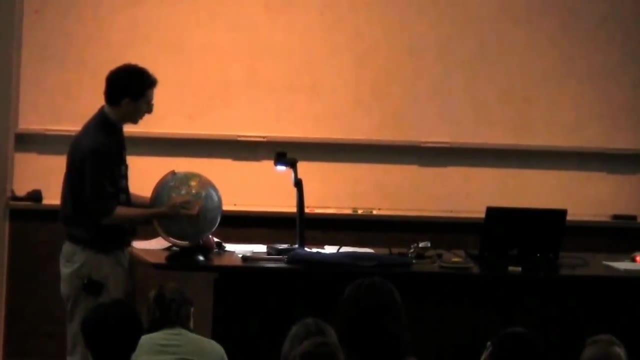 The way it works, gravitation of the Moon holds its tip in place. It can't tip back or tip in some other direction. Anyway, if we take the equator, if we take the equator of the Earth and project it off into space, 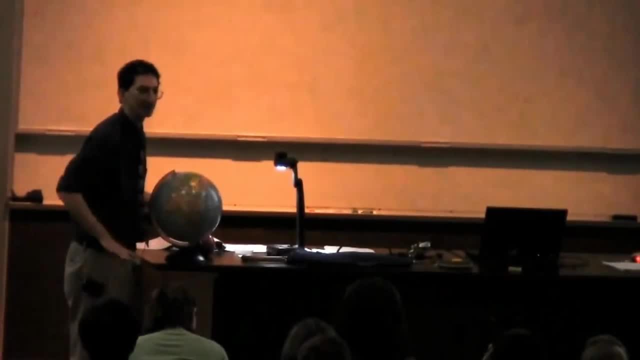 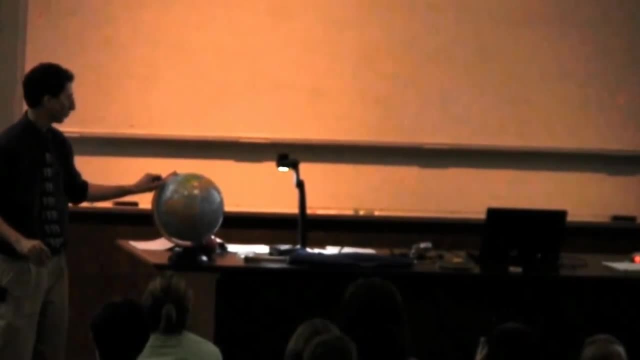 that's the celestial equator. The table is the ecliptic, the plane of the solar system. So there is a difference. They're tipped with each other by currently 23 and a half degrees. The Earth wobbles a little bit over thousands of years. 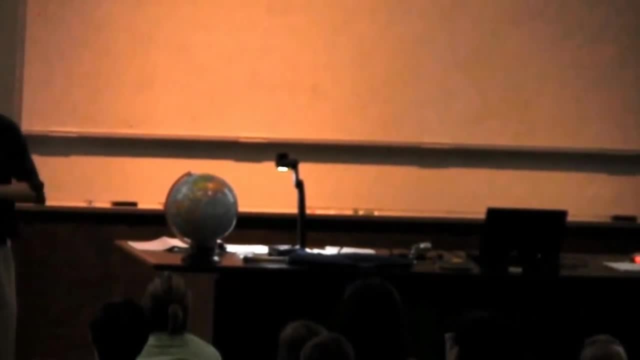 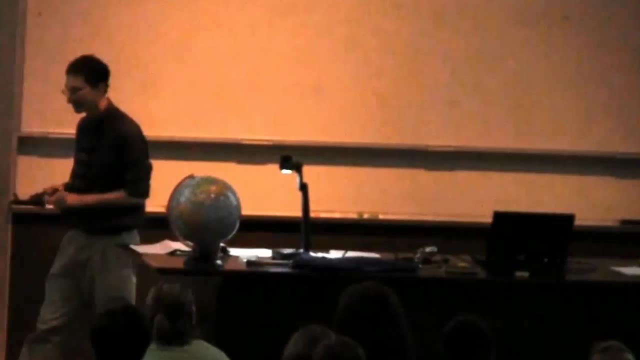 So it's anywhere between 23 and 24 degrees. Other questions: Those are good questions, Okay, So what Constellations? yeah, Let me try to wrap up constellations here For those of you who took the course. 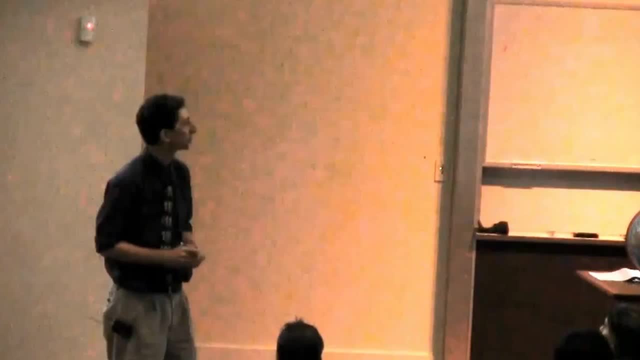 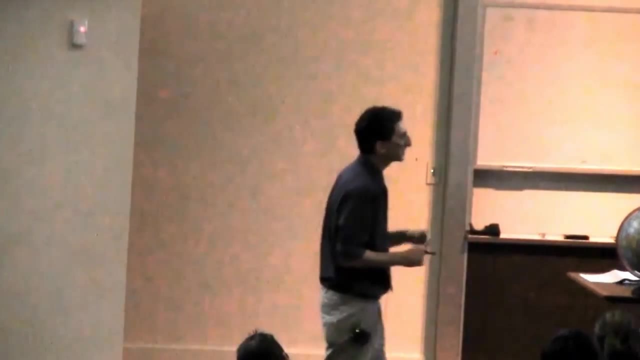 hoping to learn the constellations and learning the stories behind them. that's all good stuff, But since I only know like six constellations or seven or so, I'm not the one to teach you that, And it's better to take maybe an anthropology course, if we offer one. 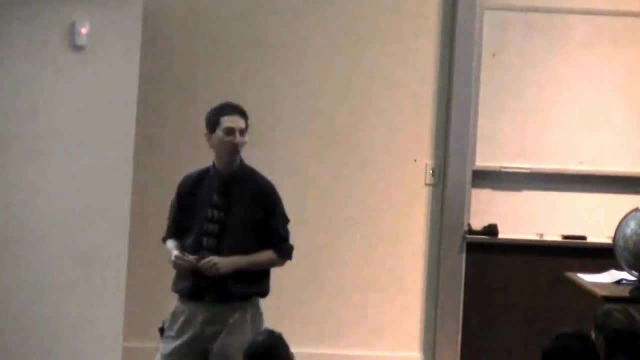 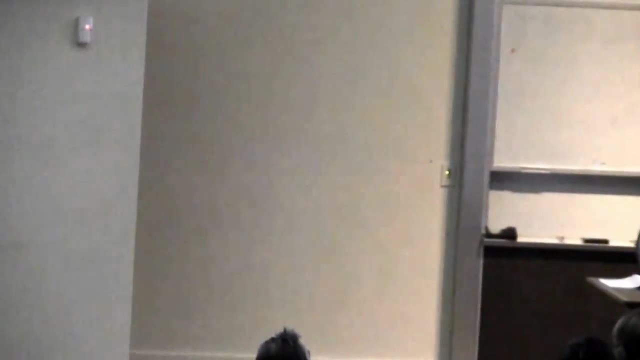 Probably don't, But the constellations tell you more about the culture, Like here. there's a collection of stars And Western civilization looked at this collection of stars and saw a guy beating a dead animal, And other cultures would see different things. 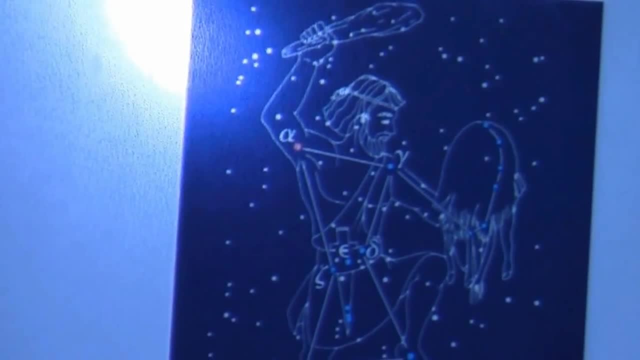 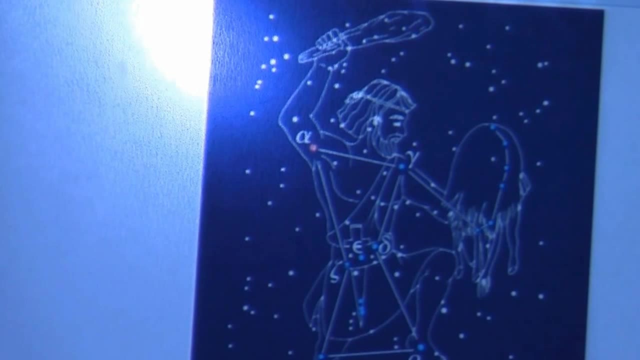 And did see different things, And it also depends on where you are on the globe. For example, if I look at Orion now, if I go outside as winter approaches, Orion will come up and I'll see this collection of stars that I might envision as a hunter. 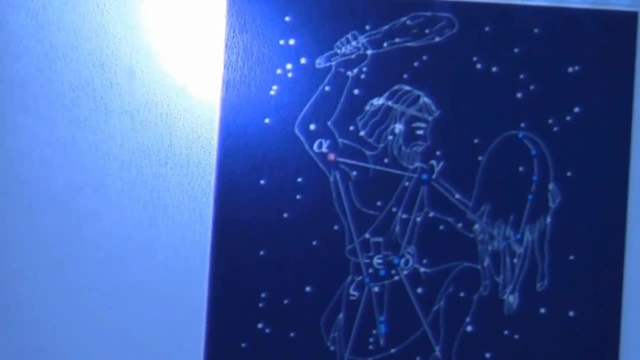 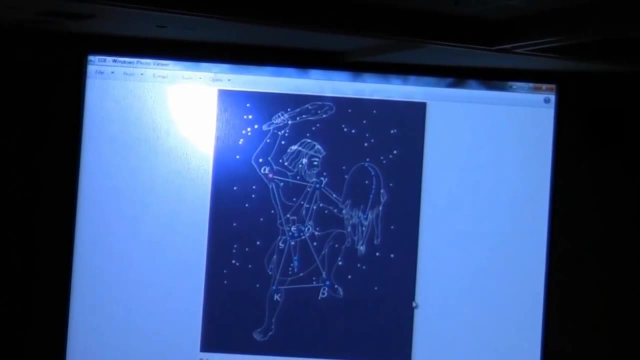 And to me it looks more like an hourglass, but they envision a full hunter and everything. But if I get- and I've actually done this- I've gotten in a plane and I've flown to Chile And this is a mid-latitude constellation. 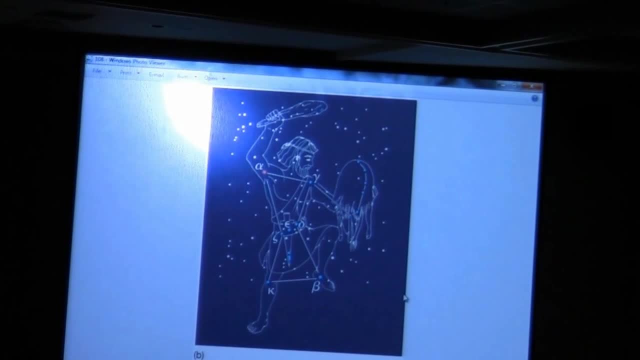 You can see it from the northern hemisphere and the southern hemisphere. What happens? as I'm flying to Chile, to this constellation? What does it appear to do? Yeah, it appears to flip over. In reality, I'm flipping over. I start out standing up. 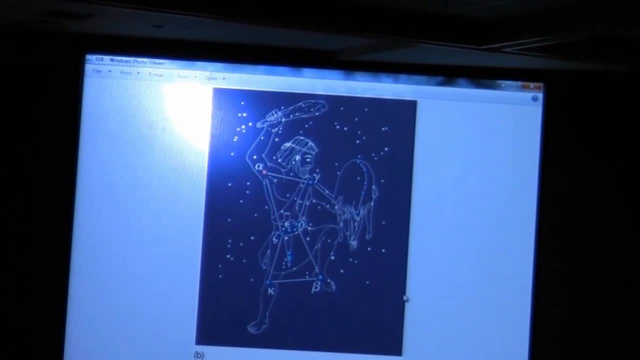 You know, up like this, looking at the constellation, By the time I get to Chile I'm upside down. So from my point of view, the constellation's standing on its head. And then, you know, people see in random patterns. 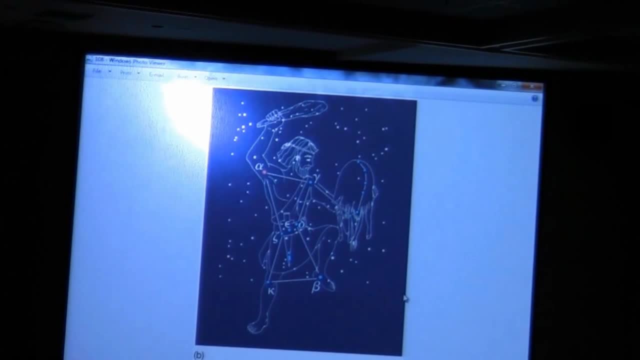 we see people, And faces in particular, all the time. It's like a psychologically proven thing. Have you ever, like stared at a rug Or a strange like? if I stare here, maybe I'll start to see it? 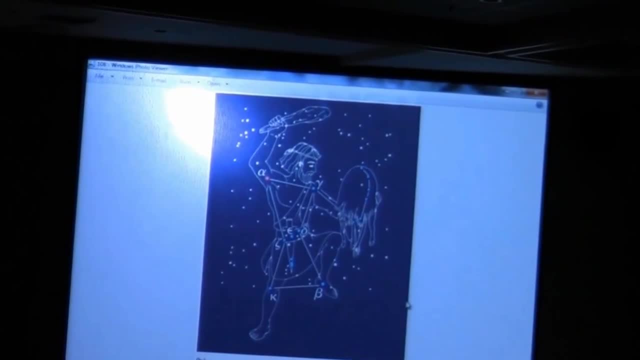 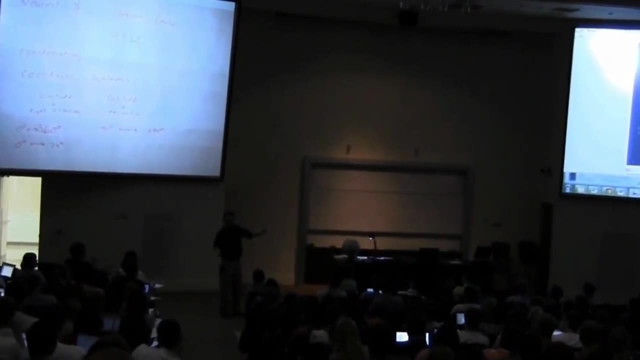 Or patterns in tiles on the ceiling or something like bored to death and just staring at the wall. Do you see like faces and people? Or is it just like my problem or something? Anyway, the brain is hardwired to see people. 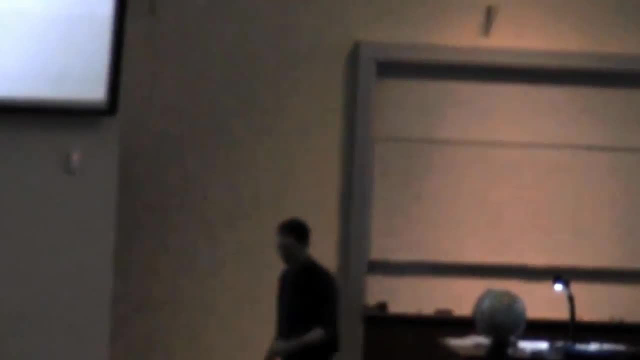 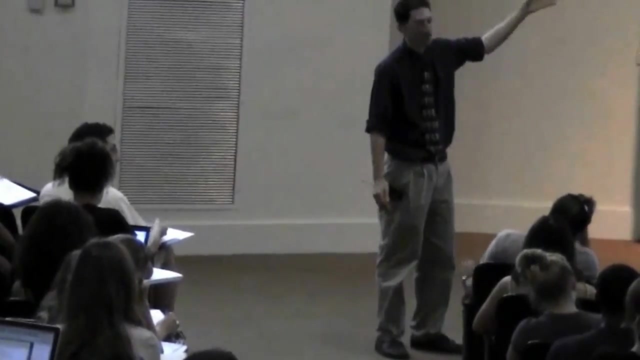 And we tend to see them standing straight up. And then see faces and we see them straight up. So if I flip this constellation, you may no longer see- And the people in the southern hemisphere never envisioned- a person standing on their head. They have different ways of connecting the dots. 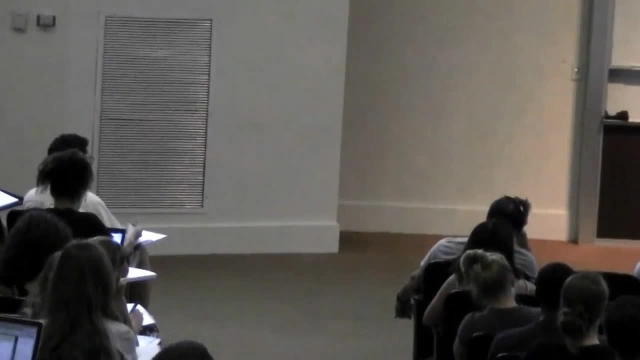 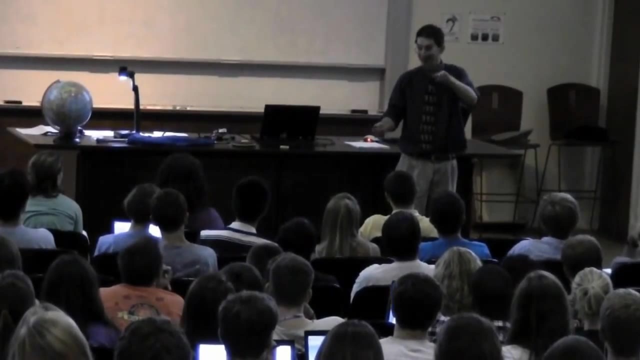 and see different things. The moon's another good example of changes with hemisphere. Have you all seen the face of the moon? Yes, I'm telling you, the brain sees faces and things Programmed to. But if we go to the southern hemisphere, 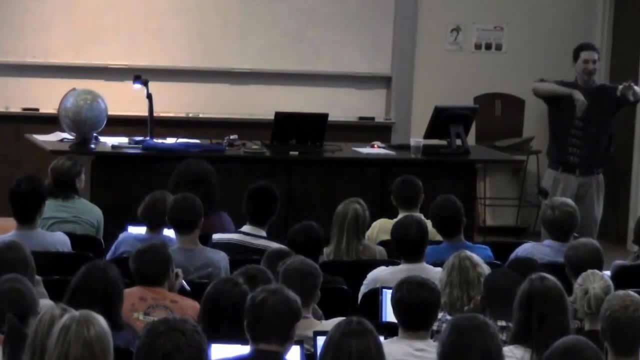 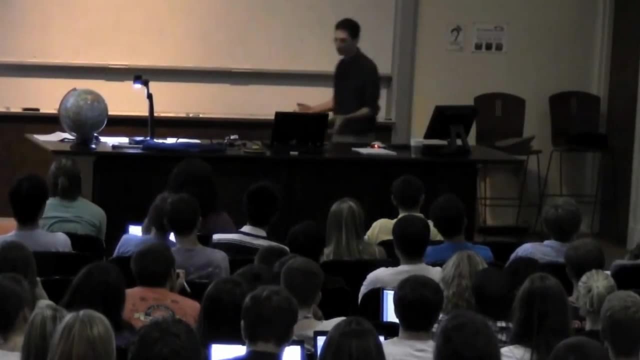 the moon is upside down. Actually, it's the same: We are upside down, We're looking at the moon standing on our head, So the splotches that make the face of the moon are now upside down, And people in the southern hemisphere 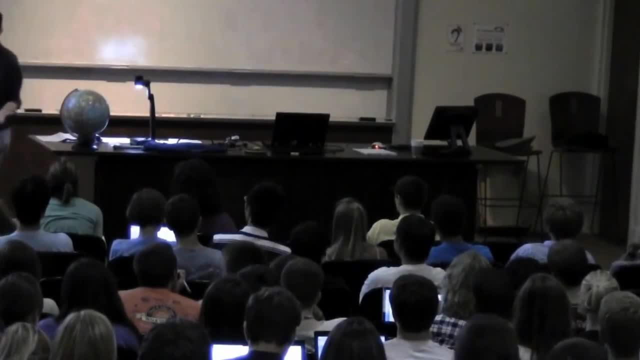 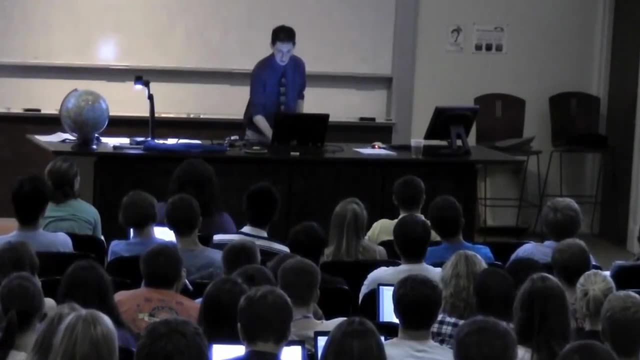 don't know what you're saying when you say the face of the moon. They're like what I've never seen: a face of the moon. Okay, I don't know what's going on here, Come on. Okay, So they're interesting culturally.